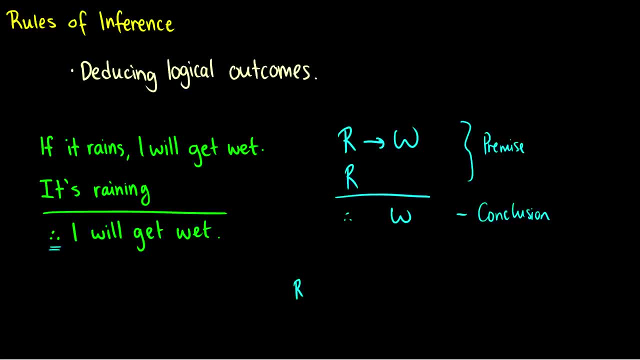 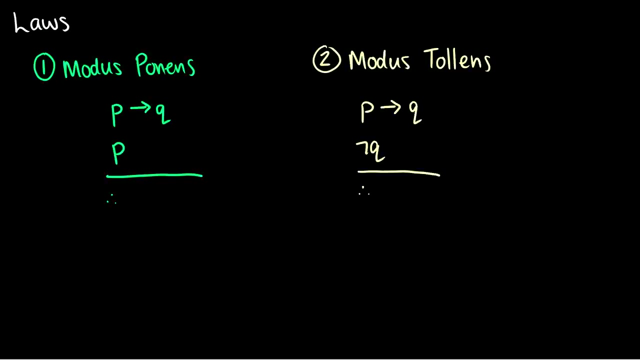 this is the same thing as R arrow W and R arrow W, And with a truth table this would be a tautology. So all of our rules of inferences of this form are going to form tautologies. So with that in mind, let's take a look at rules of inferences. So first one is modus ponens And 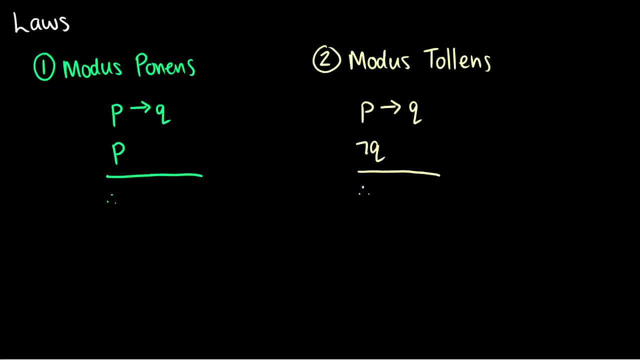 this is sometimes referred to as affirming the antecedent. So if I have P, arrow Q and I have P, then I have Q. This is like sticking the thing into the arrow and getting an output. So if we have P, arrow Q, then this says: oh, if we have P, then we have Q. Well, we have P. 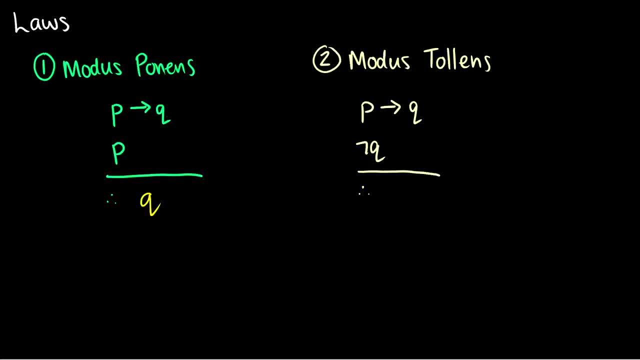 therefore we have Q Modus ponens. this is normally shortened as MPP, MPP, because this is actually modus ponendo ponens, but we just take the ponendo out because, you know, we're discrete math people, We're not philosophers. Two modus tollens: Well, modus tollens is the 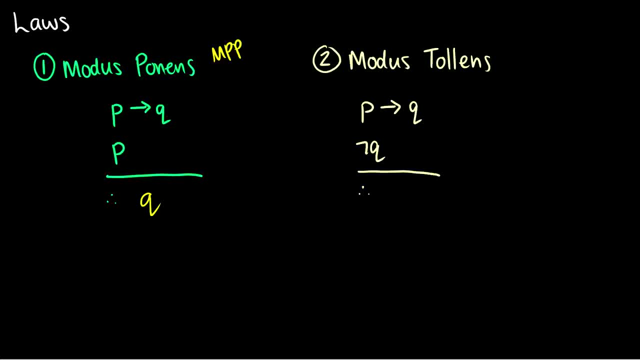 opposite way. So this is sometimes known as denying the consequent. So if we have P arrow Q and not Q, then we get not P. and if you remember, P arrow Q is logically equivalent to not Q arrow, not P. so this is kind of like doing modus ponens on the contrapositive. you can. 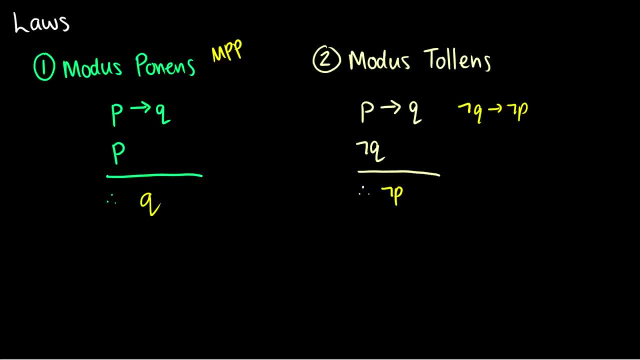 think of it like that. so if you wanted, you could just do the contrapositive law and then use modus ponens on that. that's another way of doing things, and this is sometimes shortened as MTT for modus tenendotolens. yeah, there's a. 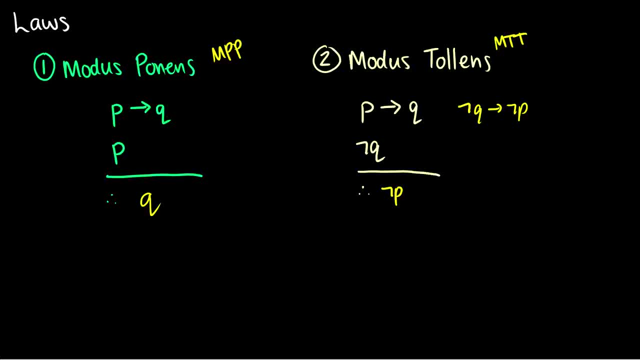 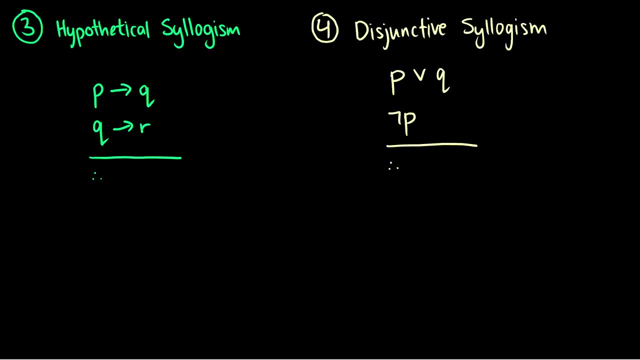 lot of tenendos and pendendos that we just removed. but MTT is the typical abbreviation, so we'll keep it like that, okay. third law: hypothetical syllogism. it's kind of like transitivity. so if we have P arrow Q and Q arrow R, then we could just say: oh, it's P arrow R were. 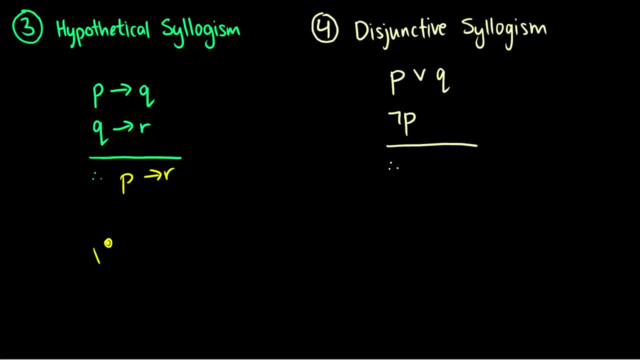 kind of like taking out the middleman. we're saying: oh, we have P and we have Q and we have R, and we have these arrows in between. we can draw those under two strategies. so here we have PC, школo-There we have. let's just take a shortcut and go straight from P to R. 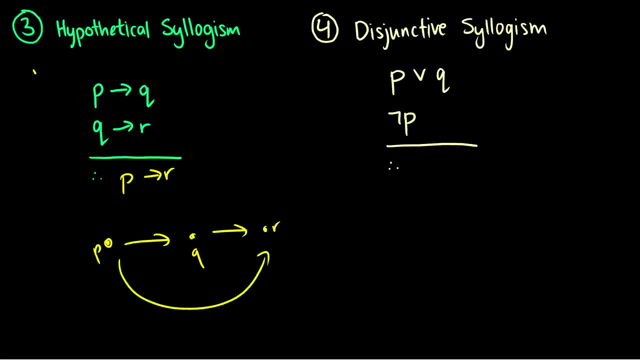 So that's what the hypothetical syllogism is and that's typically abbreviated as HS. That's just taking a shortcut, Kind of like taking these Qs and merging them together and then just forgetting about them. This one isn't typically used too often. 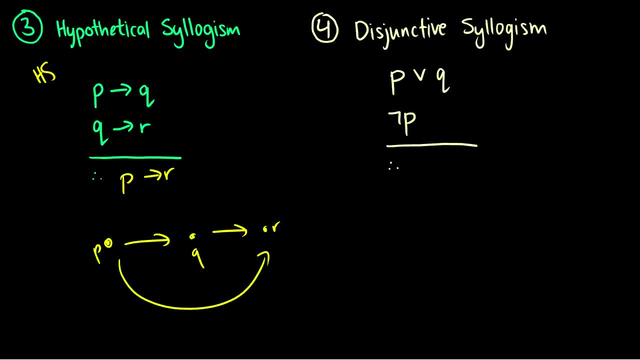 and usually we can get around this just by doing two operations of modus ponens. So if we have P in here, we can just do P, P arrow Q giving us Q, then Q, Q arrow R giving us R. Or we can shorten it by doing P and P arrow R and get R out of it. 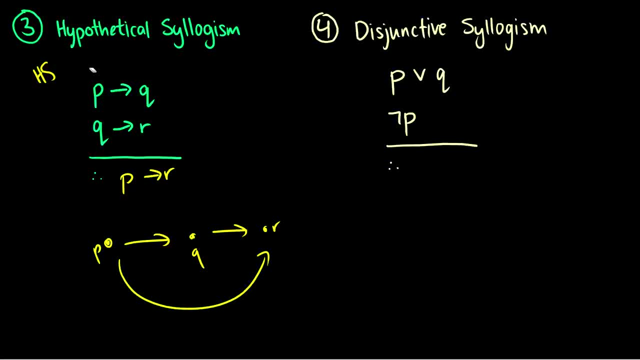 Either way works. So hypothetical syllogism isn't a required step normally. Fourth, disjunctive syllogism: If we have P or Q and not P. well, if P or Q is true, that means one of those has to be true. 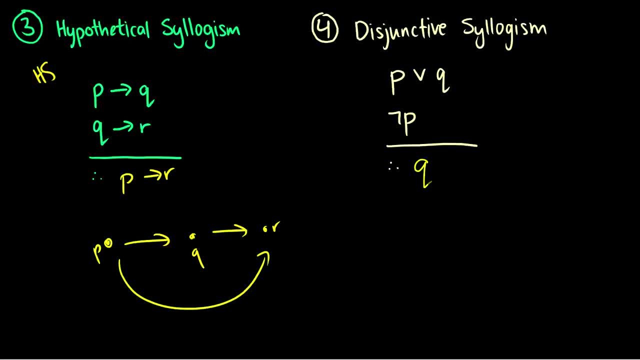 But we're saying not P. Therefore it has to be the case that Q is true And this is again abbreviated DS. So again P or Q. This says P is true or Q is true, But it's not. P says that P is false. 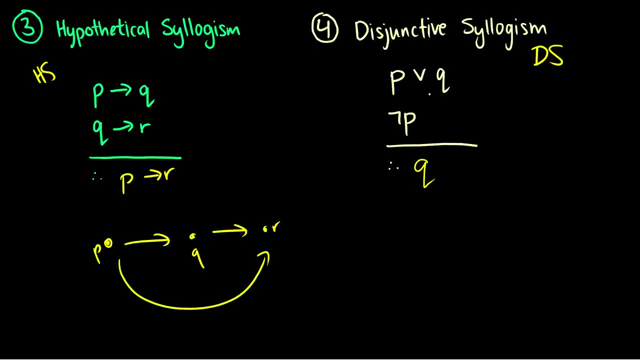 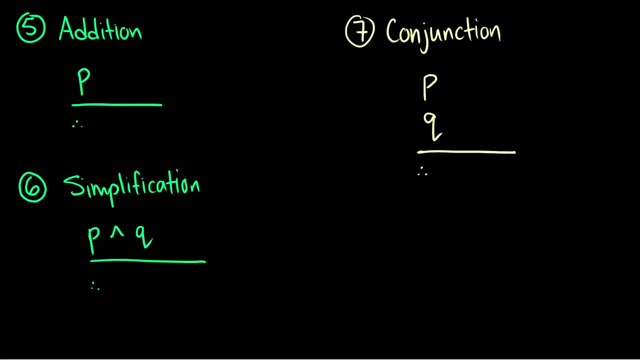 Therefore it has to be the case that Q is true. That's what disjunctive syllogism is telling us. Okay, Five addition Addition is really straightforward. If P is true, then P or Q is true. 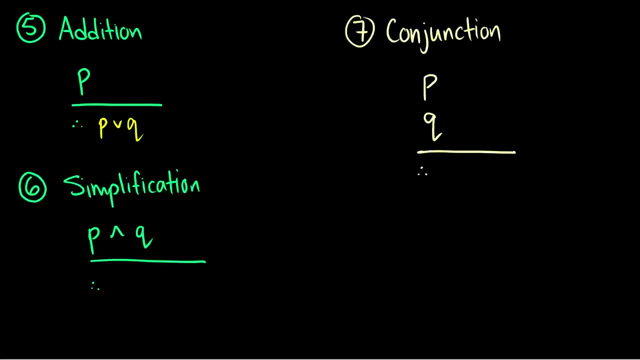 And sometimes this is just known as or introduction for VI, So or introduction, the I is for introduction And this just states: if P is true, well then P or anything is going to be true. That's just the definition of the or. 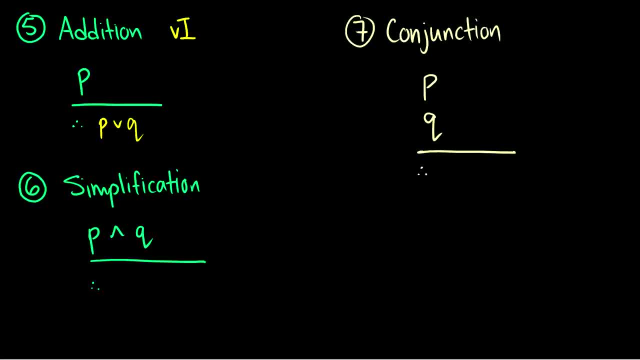 Simplification: P and Q. Well, if P and Q is true, then P is true and Q is true. Therefore, P and therefore Q. Sometimes this is also known as and elimination, because you're removing the and from it. So simplification is pretty important. 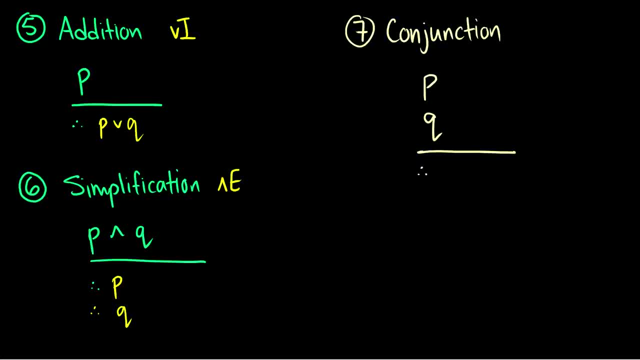 The opposite of simplification is conjunction, also known sometimes as and introduction. So if we have P and we have Q and those are both true, then of course P and Q is going to be true. So simplification is Removing the and conjunction is adding the and in between two true statements. 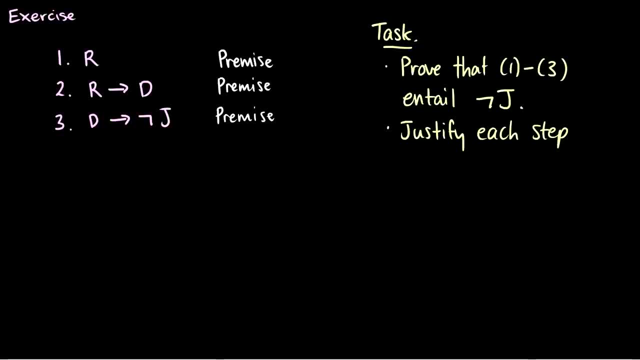 Okay, Those are all the rules of inference, that we need to do some proofs And, of course, if you remember them all, just seeing them off the first time- Wow, Incredible- Of course, I expect you to pause the video and go back and learn them and do practice with those. 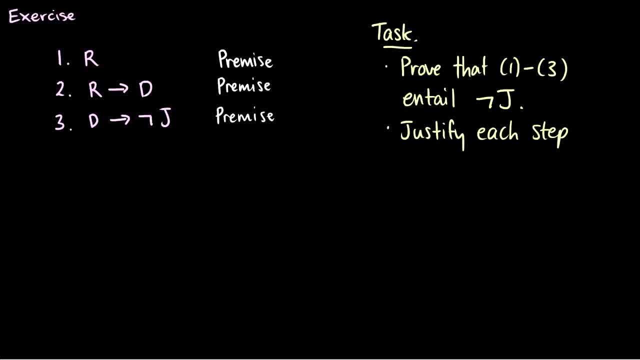 But let's just do some examples. So for the first one, I have three premises. I have R, R arrow, D and D arrow, not J, And I want to prove that one through three entail not J, And we need to justify every step. 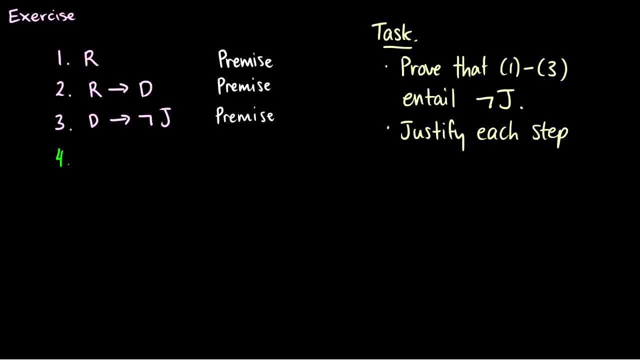 So the first thing I always want to do is I always want to do modus ponens. It's like the first thing if I see something and I see something arrow, something else, I want to stick them together. So the first one I have R and R, arrow D. 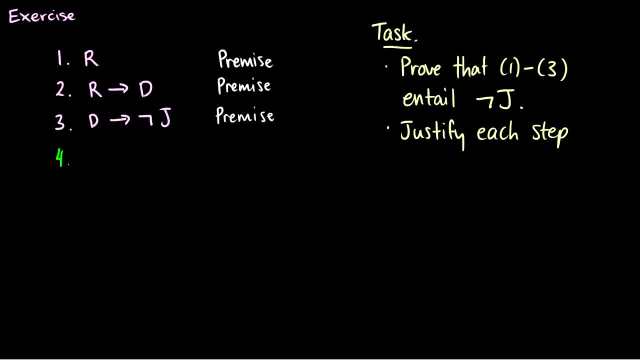 So I can do modus ponens on those and I can get D And to write a step in a proof we want to say OK. so using line one and line two we did modus ponens to get four. So from one and two we did modus ponens. 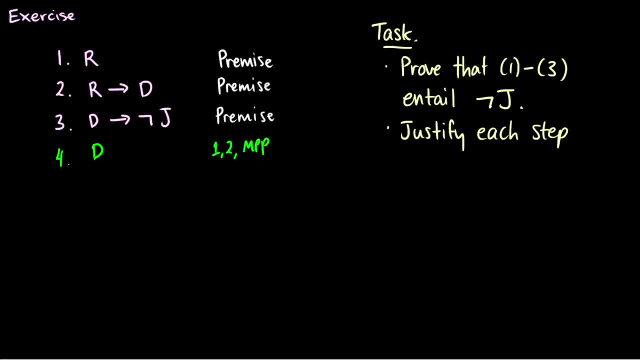 So R and R arrow D gives us D, Five. Now I have a D and on line three I have D arrow, not J. So through modus ponens I can get not J Using three, four and modus ponens. 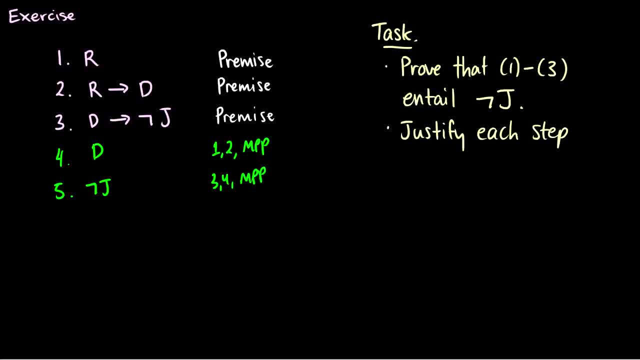 So we have shown, using our three premises, that we can get not J. Now, of course, that wasn't the only way to do things. We could have used hypothetical syllogism. So, using two and three, we could have merged R arrow D and D arrow J together to get R arrow, not J. 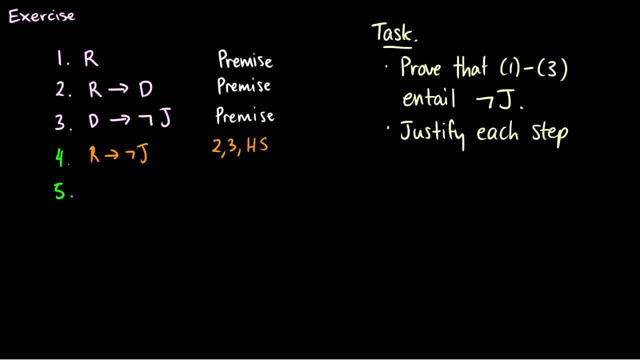 Using hypothetical syllogism, And then we could have applied modus ponens on lines one and four. So two different ways to do the same proof or to get the same conclusion. Let's do one more example. So I have not R or not F arrow, S and L. 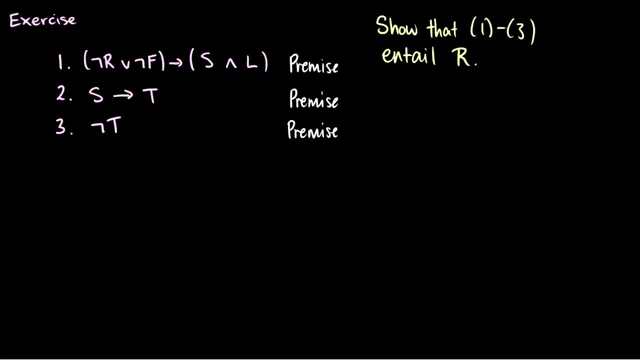 I have S arrow, T and not T, And I want to show that R, And right away you're saying: whoa, This isn't just modus ponens, What's going on? Yeah, it's not always super straightforward, But what do we see? 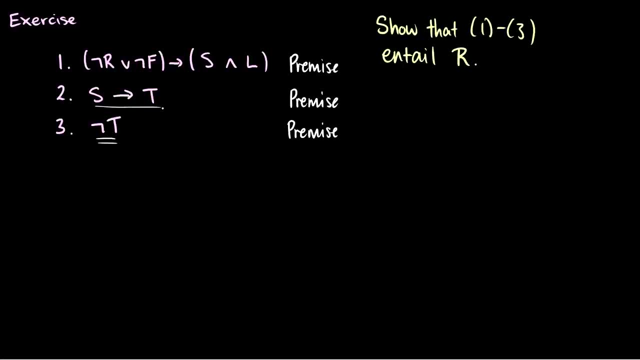 Well, we see not T and we see S arrow T. So I think this is a good time to use modus tolens. So if we have S arrow T and not T, this means we get not S. So this is two, three and MTT. 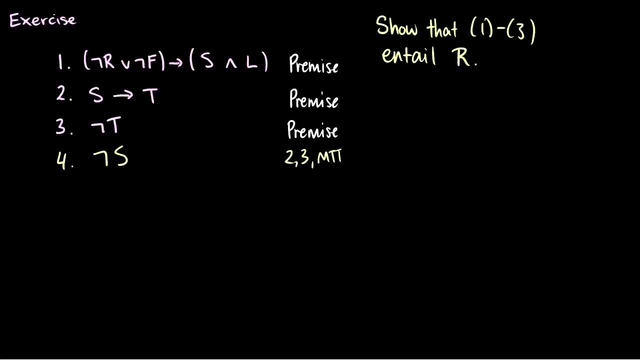 So now we have not S And we're thinking: what can we ever do with this? Well, in line one, what we could do is we could just use the conditional law and see where that gets us, Or we could take maybe the contrapositive of one. 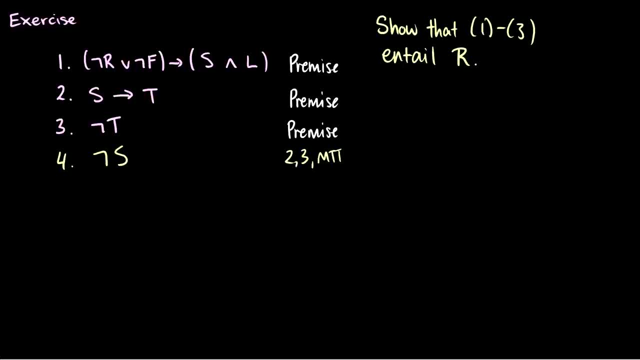 So again, we can still use our logic laws if we want. That's still available for us. So the logic laws. with the contrapositive we would get not S and L arrow, not not R or not F. OK, and this is just line one. 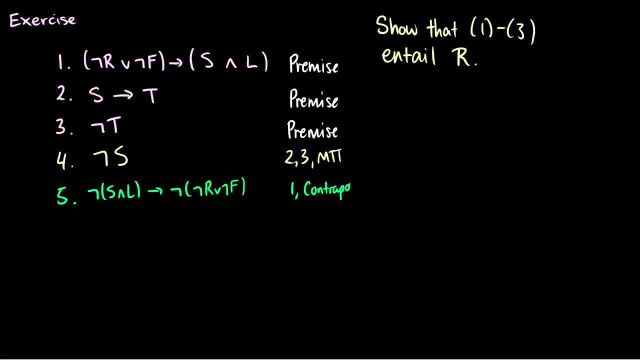 And this is just the contrapositive. OK, so now we're a little bit closer, So let's use another logic law that we have, Let's use De Morgan's law on both sides of these, So we'll have not S or not L from using De Morgan's on the antecedent. 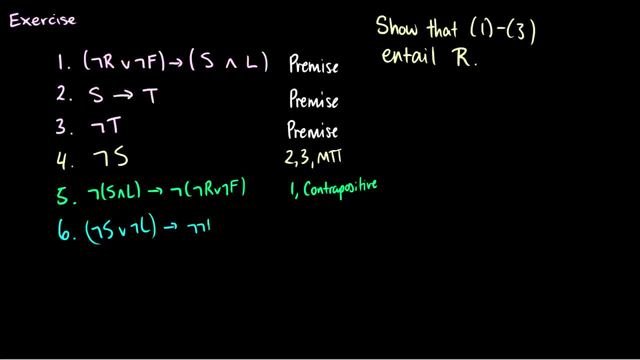 And then De Morgan's on the consequent will give us not not R and not not F. So that's on five and that's, using De Morgan's, OK seven. Well, let's use double negation Just to make things look a little bit nicer on the right side here.